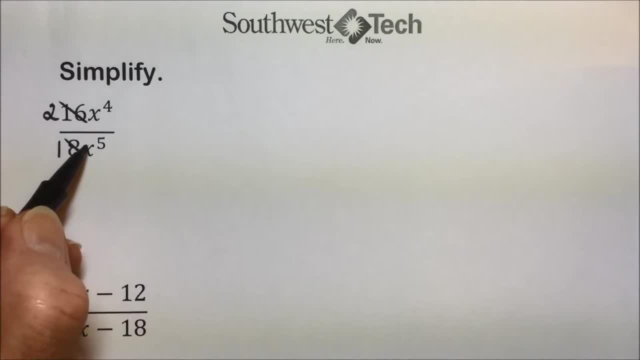 divided by eight leaves a two. We have common bases of x as well with the greater power in the denominator. so we'll do the subtraction of our exponents because of the division in the denominator to avoid a negative exponent. If we had done four minus five we would have had x to the negative. 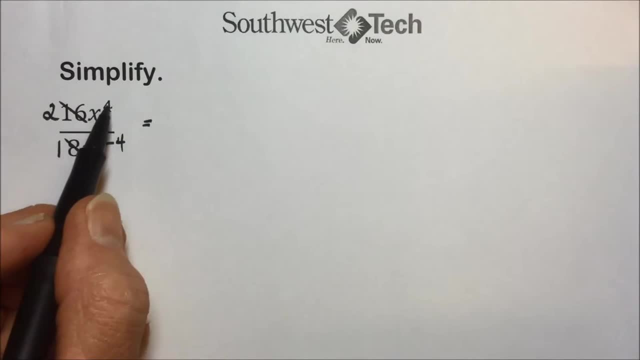 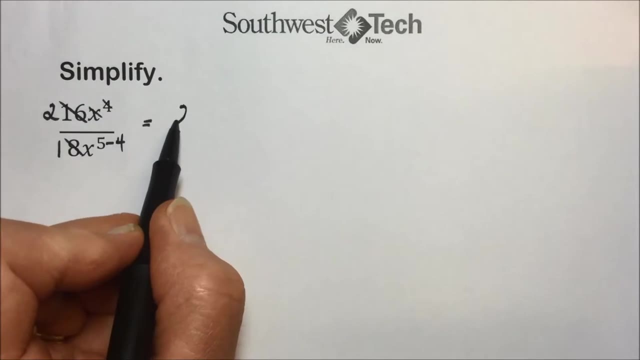 one. Instead we'll leave our x in the denominator. So the x to the four actually is cancelled out because we're doing the subtraction of exponent down here. Our numerator only has the two And we reduced our sixteen over eight And the denominator x to the five minus four. 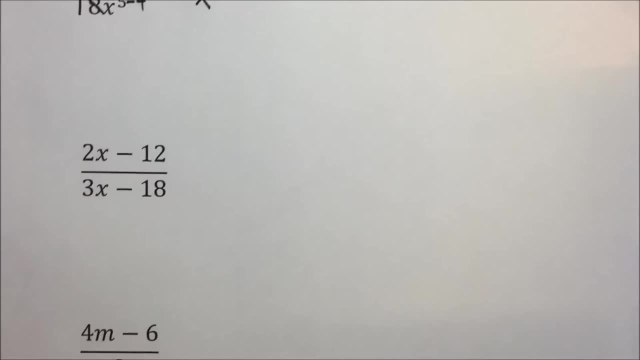 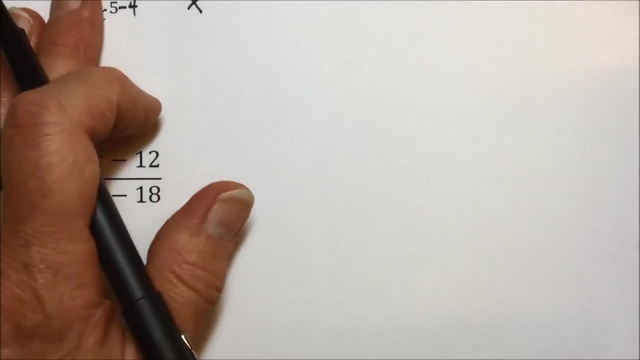 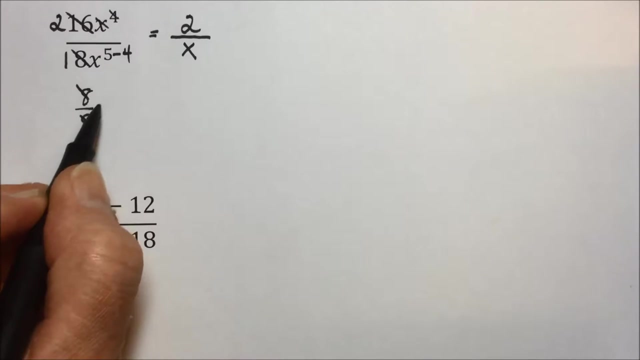 leaves us with x to the first or just simply x In this next problem. when we're reducing, we're looking for common factors that cancel out. Just up we had in this previous example. we had an eight over eight which cancelled out, leaving us with a one because it was. 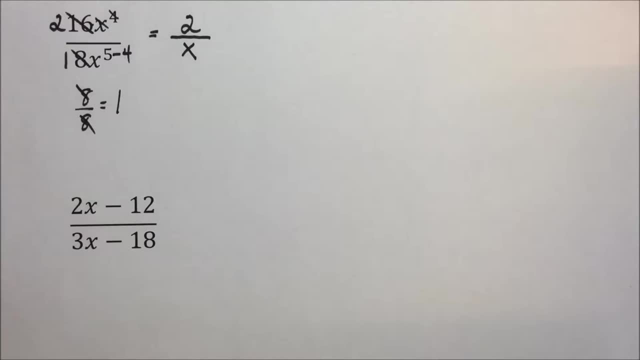 a common factor, something that was multiplied together. So the denominator here was one over eight And we reduced the exponent by a normal factor. When we look at the denominator, it's a two over nine. Now you might say to yourself: I don't guess you can figure that out. 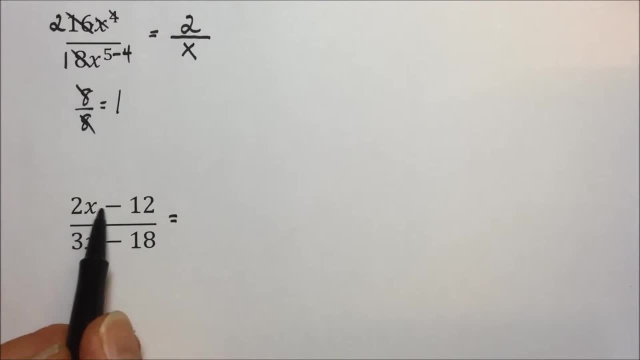 Yes, you can, But you can't really circle back and forth. That's right, You can't really circle back and forth. It's just a matter of the number of factors. So one over eight is the two over nine, which is always the same, but it's the same number. 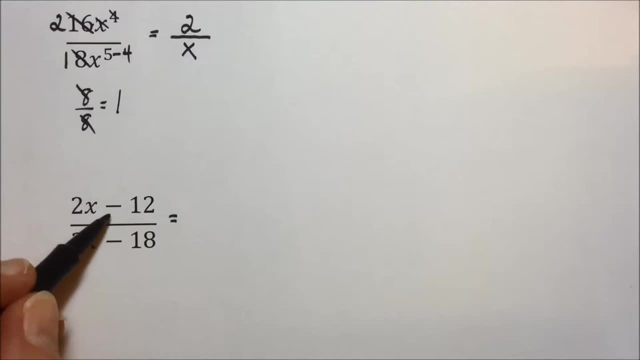 over nine when you're in the denominator And the denominator is a constant. So this is fine. I'm not sure how I'm going to divide that into a number. We'll look at that later. So when we're done with looking up and down, we're going to go into the denominator. 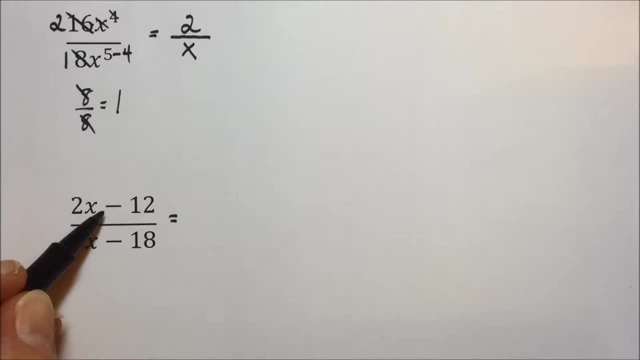 With an addition or subtraction, in this case the subtraction. there's nothing that we can do as far as reducing this until we have a product of factors. So in the numerator common between the two terms is a greatest common factor of 2.. 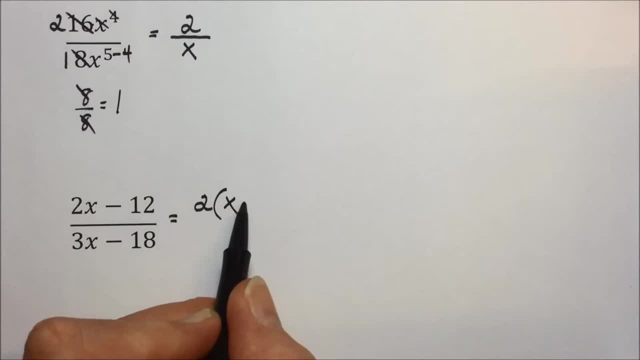 2x divided by 2 leaves an x Negative. 12 divided by 2 leaves a negative 6.. We now have a product of two things: a monomial and a binomial. that's equivalent to this original expression. Similarly, we'll factor the denominator. 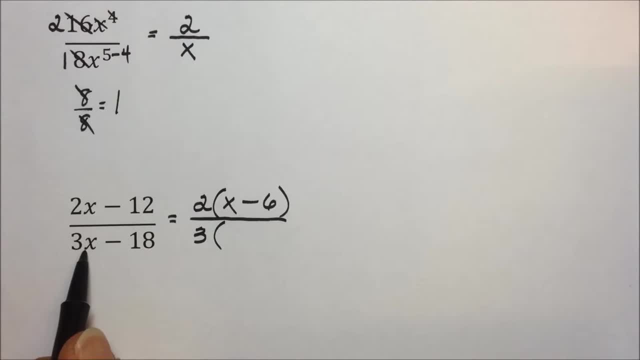 Greatest common factor is a 3. Dividing or factoring by a 3 leaves an x for the first term, And negative 18 divided by 3 leaves a negative 6.. Now we'll look in the numerator and the denominator and if we see a common factor that cancels out, we'll do so. 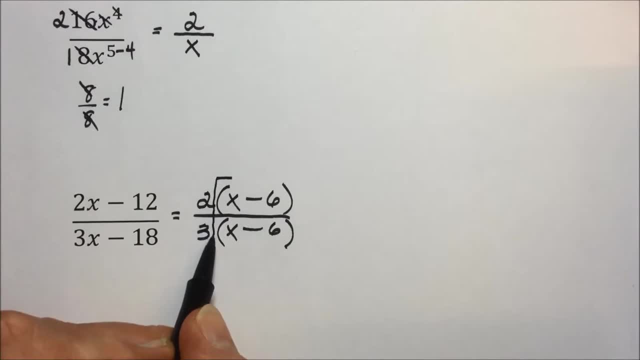 And if we look, 2 and 3.. 2 and 3 don't have anything common, but we do have a common binomial in the numerator and the denominator, just like an 8 over 8 cancelled out to equal 1.. 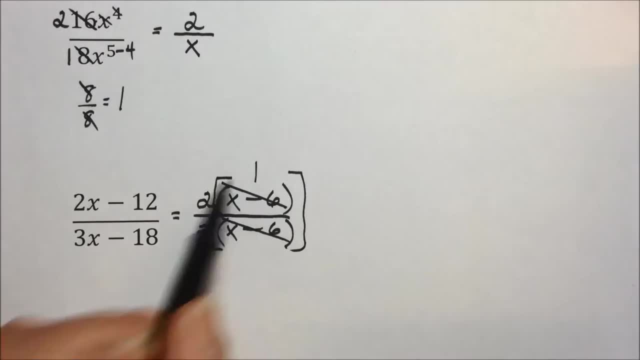 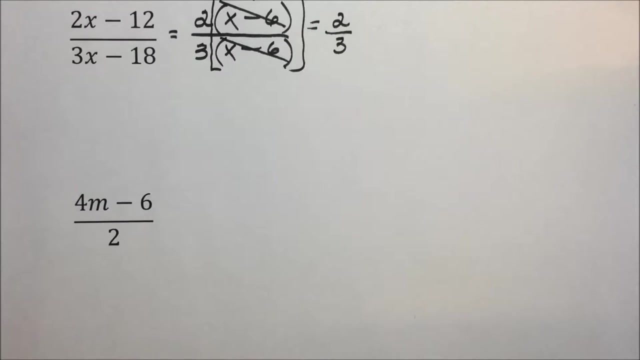 An x minus 6 over an x minus 6 cancel one another out, leaving a 1.. 1 times 2 thirds leaves us with a final answer of 2 thirds for the reduction of this rational expression, If you recall, from adding and subtracting. 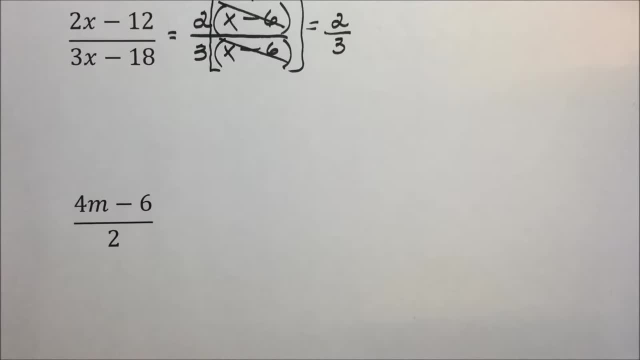 fractions together, we have to have a common denominator. And this is going to help us when we have a polynomial divided by a monomial or this rational expression. To simplify it, we're going to use the following concept: When you add fractions or rational numbers together, you have to have a common denominator. 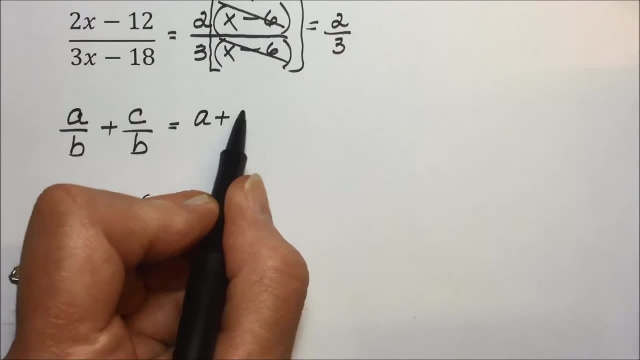 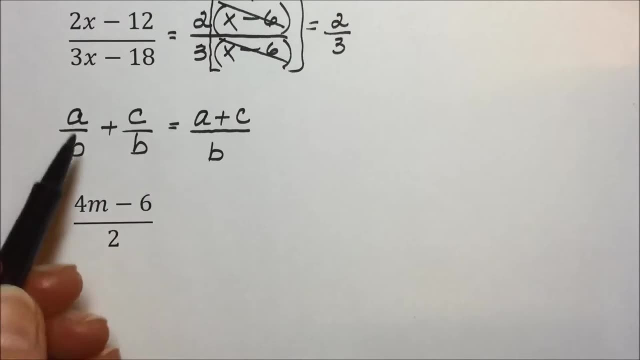 Having a common denominator, you then go ahead and add the numerators over that common denominator. Generally, we're going from left to right, adding common denominators or adding fractions together that have common denominators, giving us the final result, But we're 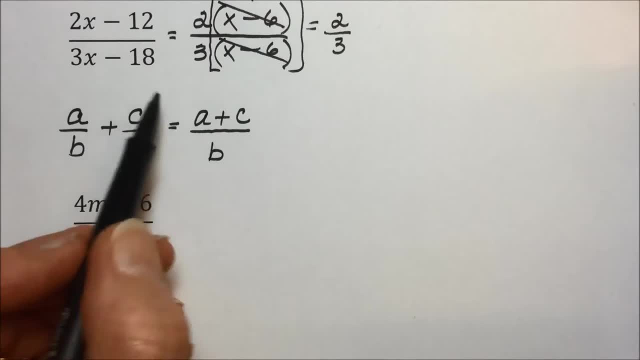 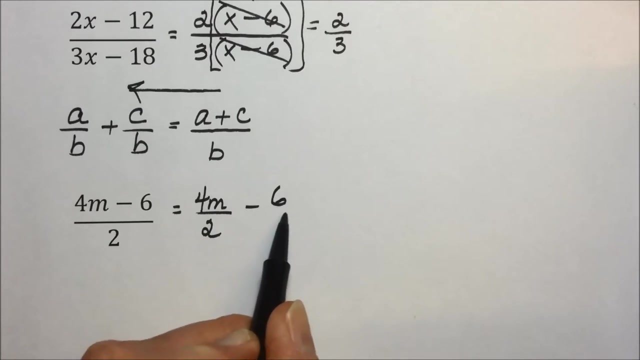 looking at an expression that's similar to this right-hand side, and we're going to reverse this direction. Where did this rational expression come from? Each of these terms must have had that common denominator, which, in this example, is 2.. So we're going to pull those apart. 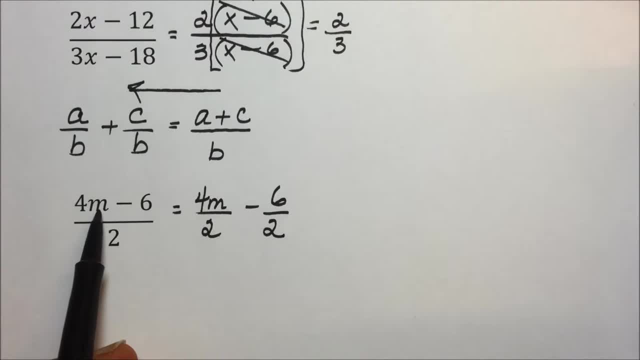 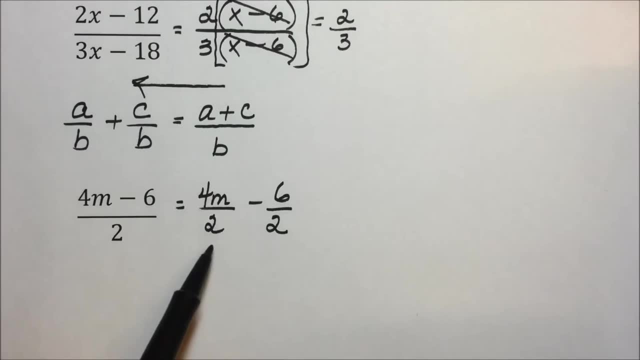 Common denominator, you would combine your numerators and that's what we have. but by pulling them apart we now can simplify each of these rational terms here: 4m over 2, or 4 divided by 2, is going to leave us with a 2m, because 2 divided by 2 is 1.. 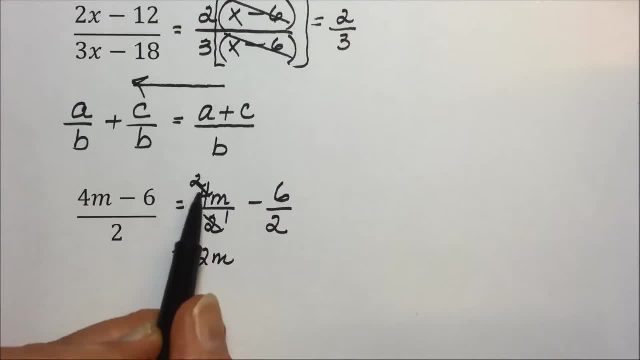 4 divided by 2 is 2,, and 2 times m leaves us with the 2m over 1,, or 2m minus 6 divided by 2,, or divide the numerator by 2, leaves a 3.. 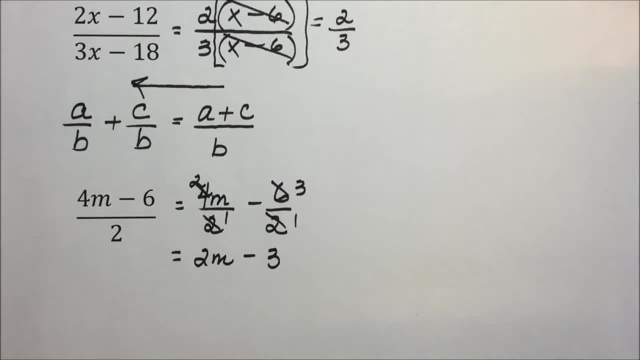 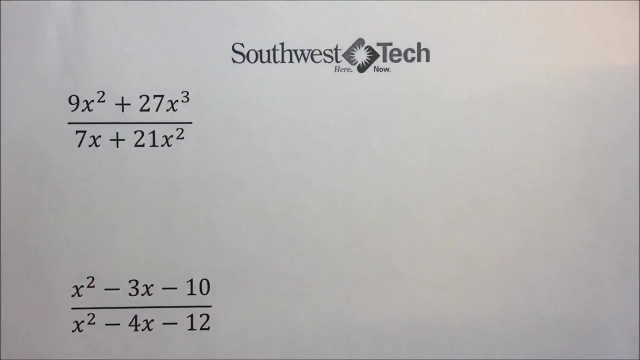 Divide the denominator by 2, leaves a 1, and 3 over 1 is a 3.. So we've reduced our rational expression by going to the undoing of our common denominator when adding or subtracting fractions or rational expressions. 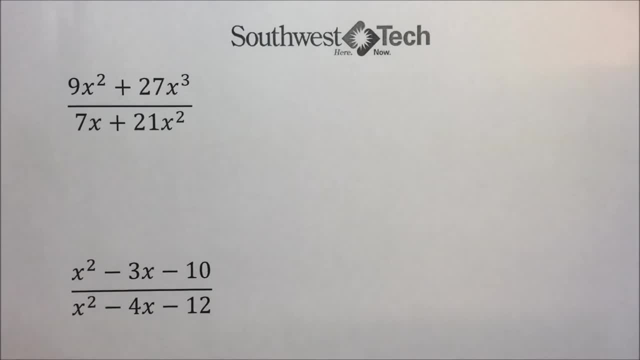 They're asking us to simplify here as well. and again, caution you before looking numerator denominator to cancel terms out factor instead, because you're looking for a common factor. So in the numerator greatest common factor between those two terms is a 9 for the integers. 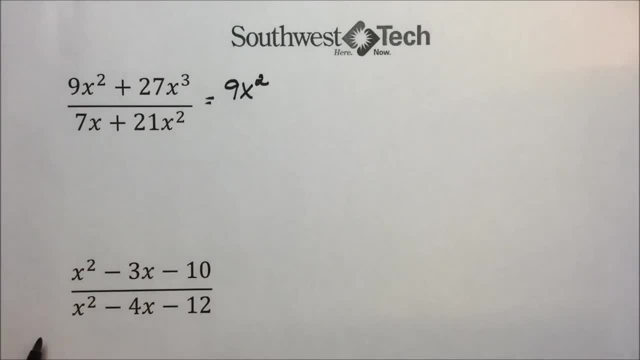 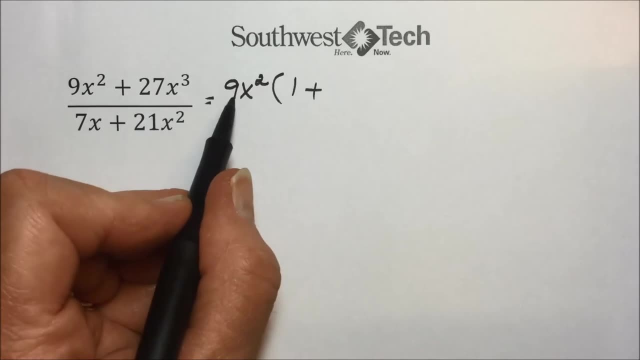 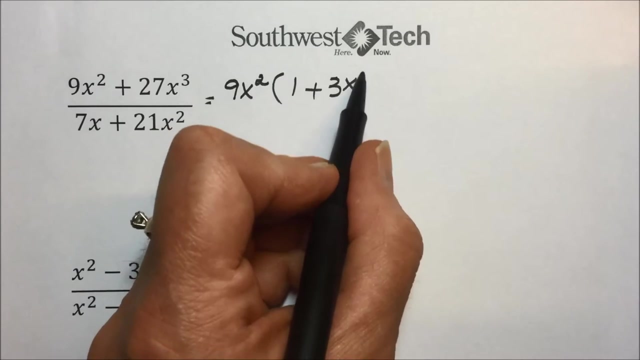 and an x squared, the lowest common power between the two terms. dividing the first term by 9x squared leaves a 1, 27x to the third divided by 9x squared. 27 divided by 9 is 3,. x to the third over x to the second leaves an x. 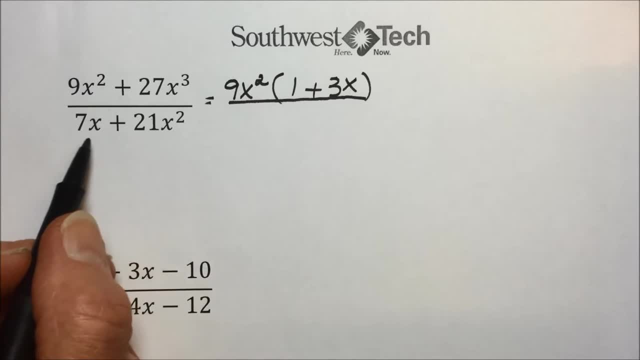 In the denominator greatest common factor is a 7 in terms of the integers and an x for the variables. It's the lowest common factor, It's the lowest power common to both of those terms. Factoring is dividing, so 7x divided by 7x leaves a 1, 21x squared, divided by 7x leaves: 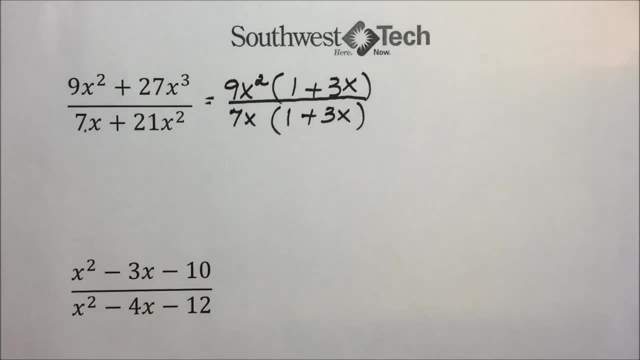 a 3x. Now we can look numerator and denominator. what are the common factors to the numerator and the denominator, canceling out anything common? We have an x plus 3 over an x plus 3, which is 1, the most obvious one. 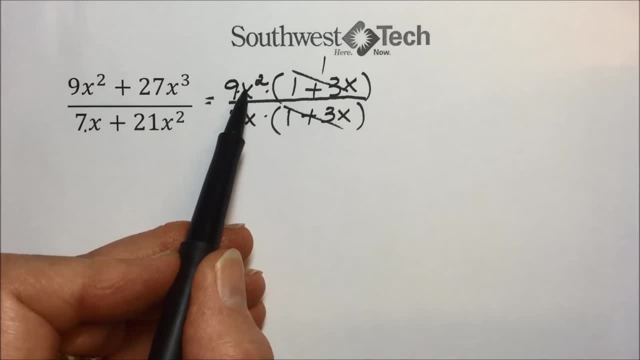 9 and 7 don't have anything common, but x's are common common bases. subtract our exponents 2 minus 1, since the higher exponential powers in the numerator leaves us with an x to the first in the numerator and cancels out the x in the denominator. 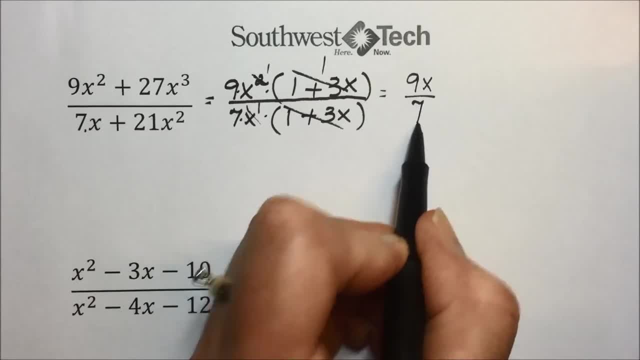 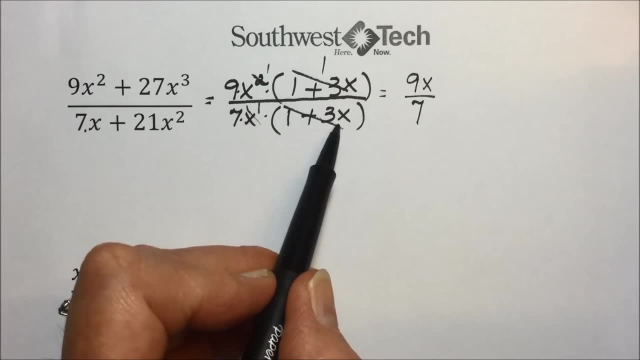 Final answer, then, is a 9x over the remaining 7.. Always, it's a good idea, when you factor, to be sure you multiply distributively: 9 and 7 don't have anything common but x's are common. or FOIL method, if appropriate, to be sure that you have an equivalent expression before you move. 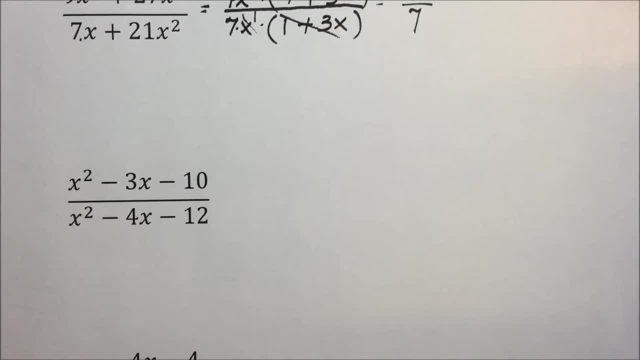 forward. In this next one, again, we don't have any common factors because these terms are connected with subtraction, so we can't cancel out yet. but if we factor, perhaps we will find a common factor. We're looking for numbers that multiply to give us negative 10 and add up to be a negative 3. we 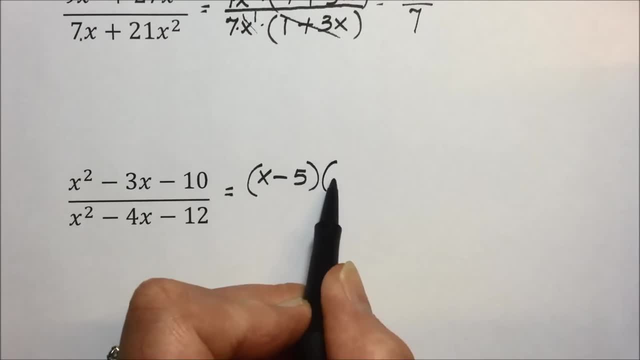 don't have a lot of choices and the pair that works is an X minus 5 and an X plus 2. in the denominator we're looking for factors, two binomials that multiply together to give us this trinomial, and we're looking at, specifically, factor pairs that multiply to give us negative 12. 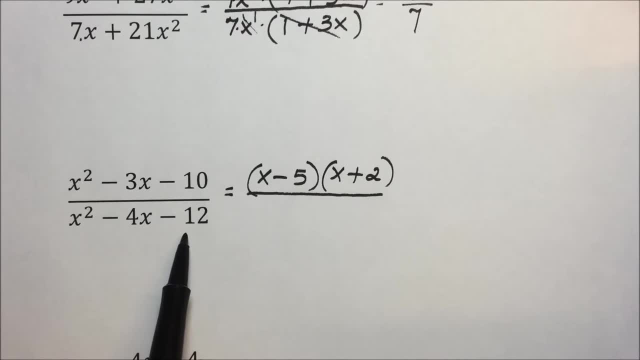 and add up to give us this trinomial, us a negative 4.. We have several choices: 1 and 12,, 2 and 6,, 3 and 4.. One has to be positive and one has to be negative, And the pair that works is an x plus 2 times an x. 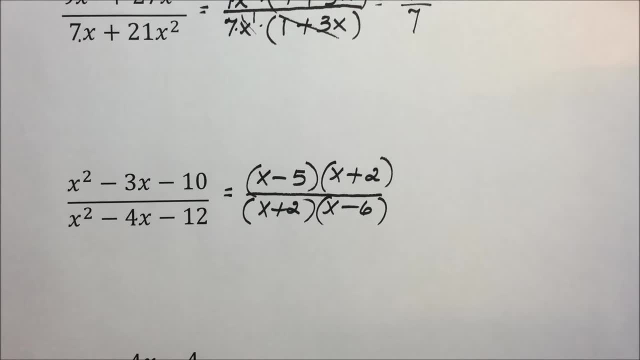 minus 6.. Again, always check your factoring. multiply them back together to be sure that you have an equivalent expression. Now we have factors, something times something in the numerator, likewise in the denominator. that we can look in the numerator and the. 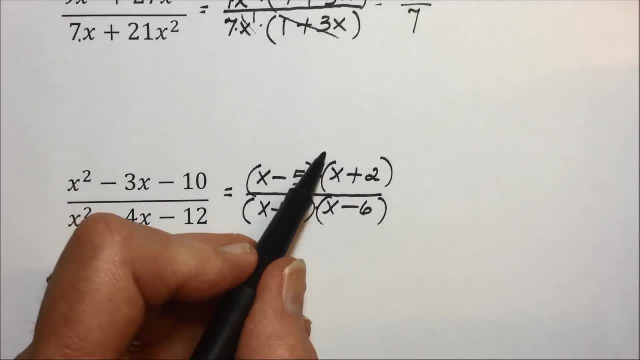 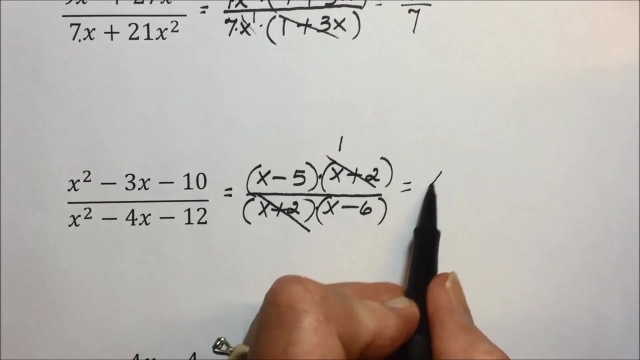 denominator for a common factor. There is an x plus 2 in the numerator over an x plus 2 in the denominator. That is equivalent to a 1.. Anytime you have the same quantity over the same quantity, it reduces to a value of 1, leaving us with an x minus 5 over an x. 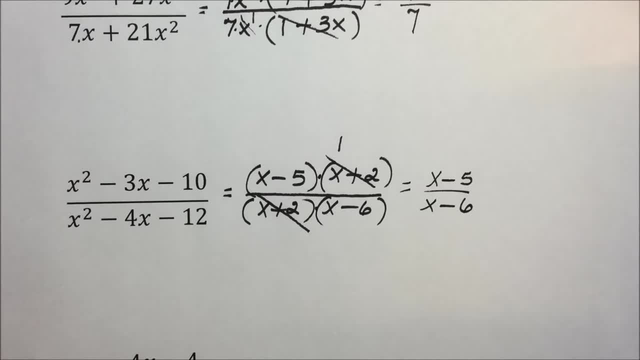 minus 6.. That is our final question Answer, And we have to know when to take the breaks off. You may be thinking, but there's a common x. These are not connected with multiplication, so we have to stop there. Only if we had that. 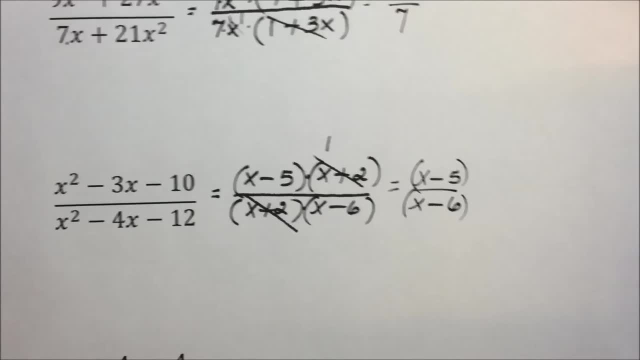 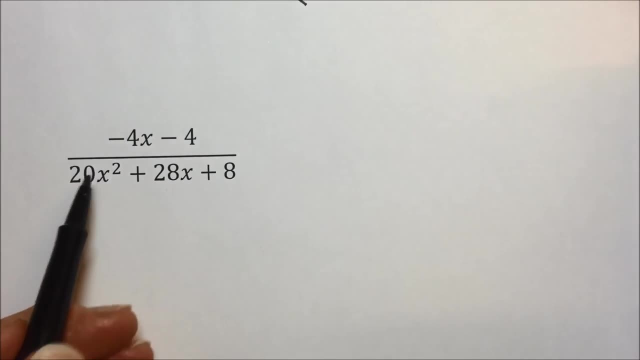 similar binomial in the numerator and denominator. could we cancel it out? This last example? they're asking us to simplify or reduce this Again. we start with factoring the numerator, Do not look up and down for common factors. yet We don't have factors. 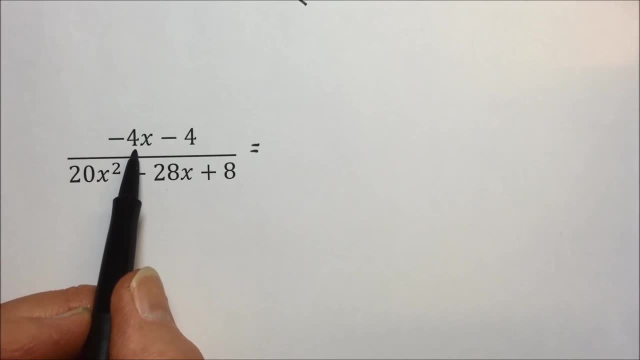 So between the two terms there is a 4.. And just because we normally have positive x's on our factoring in our binomial, let's take out a negative 4 in anticipation of not leaving a negative x. Instead, factoring out a negative 4 will cancel out the negatives and leave. 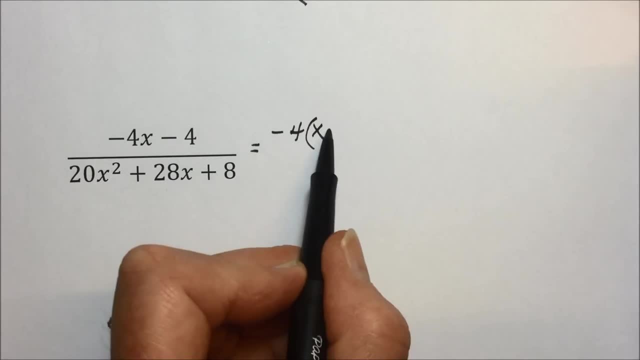 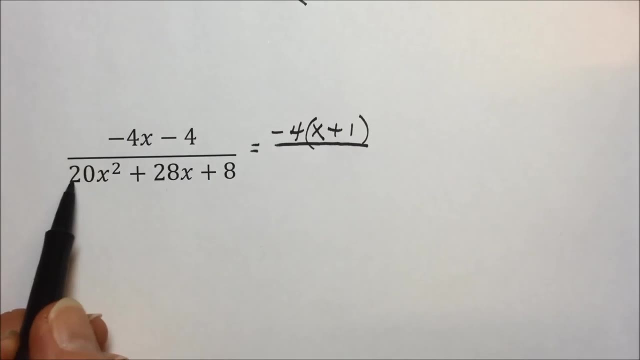 a positive x. Negative 4 divided by negative 4 will leave a negative x. So we have a negative, positive 1.. Distributively we can see we have what we had In the denominator. there's definitely a common factor of 2. And if we dig a little deeper we find there's a common 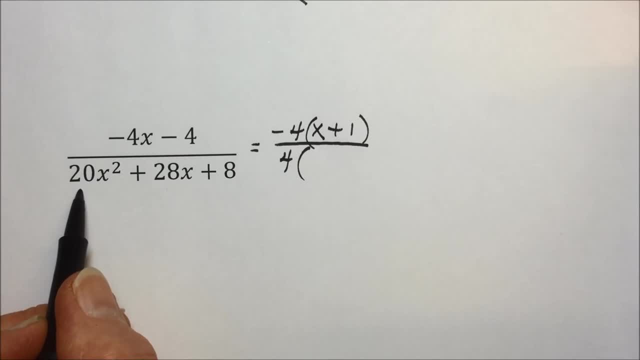 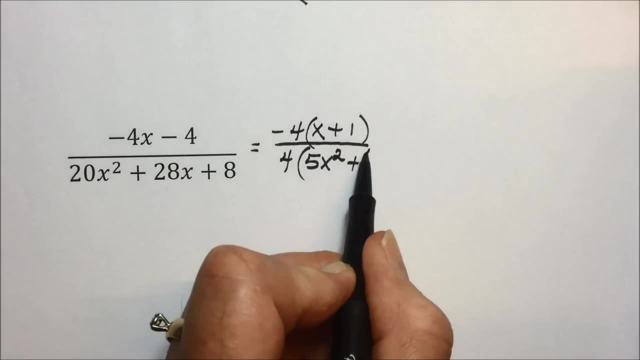 4. Each of these terms divided by or factored out. factoring out a 4 leaves us with a 5x, squared a 7x and a 2.. Right now, we have two things multiplied together in the numerator. 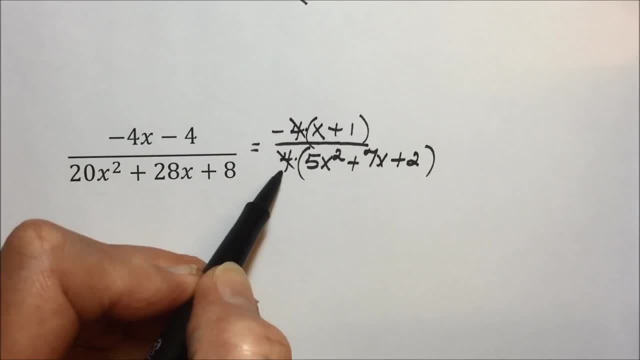 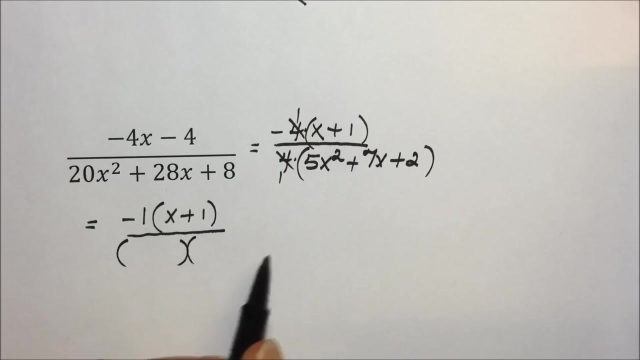 and the denominator with a common factor of 4.. So the 4's cancel out, leaving a 1.. So we have a negative 1 times x plus 1 in the numerator. In the denominator, we have this trinomial left which- let's see if we can factor it, 5x squared- must have come from: 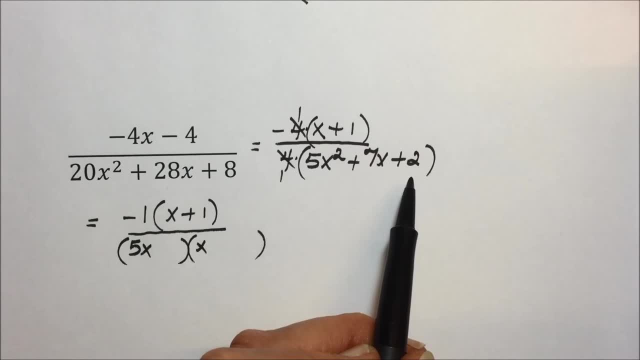 a, 5x and x Two. we don't have any choices other than 1 and 2.. Both signs are the same, Both are positive, But we have two options of where we put that 2.. We can put it here: 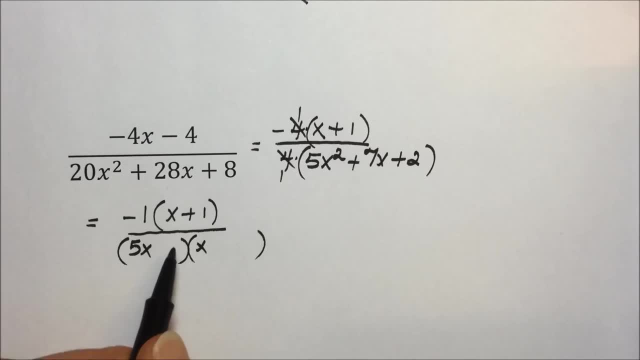 So we would have a 2x and a 5x, which do add up to be the 7x. Or we could put our 2 here, which would have given us a 10 and a 1, which would not have given us the 7. So a 2 here. 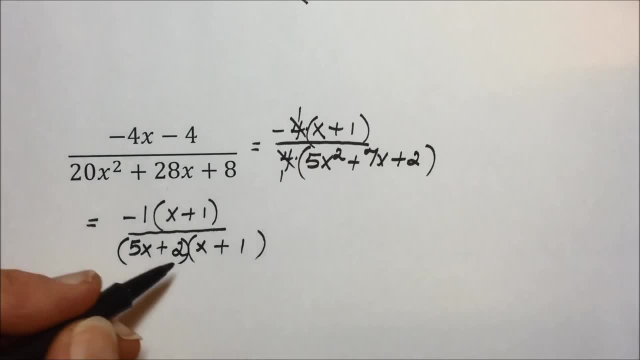 and the 1.. Now, looking again, we have more factors And we have in the numerator and the denominator an x squared. So we have an x squared plus 1 over an x plus 1, which cancels out. So our final answer: 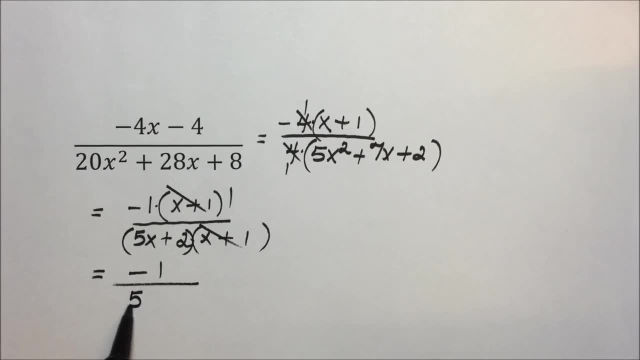 leaves us with a negative 1 in the numerator and this binomial 5x plus 2 for the simplified form.